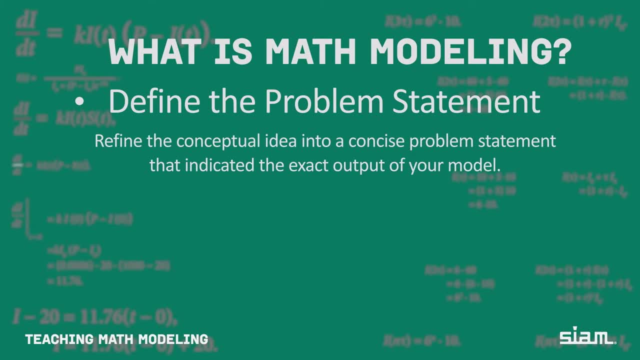 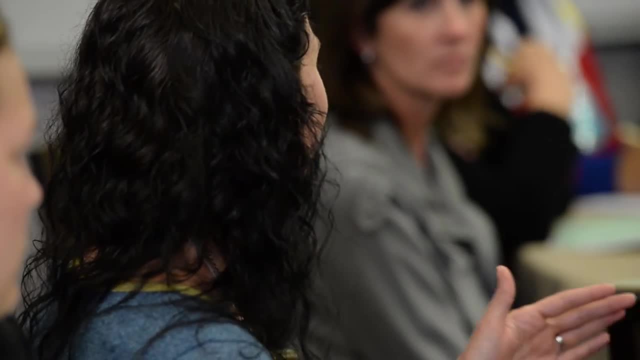 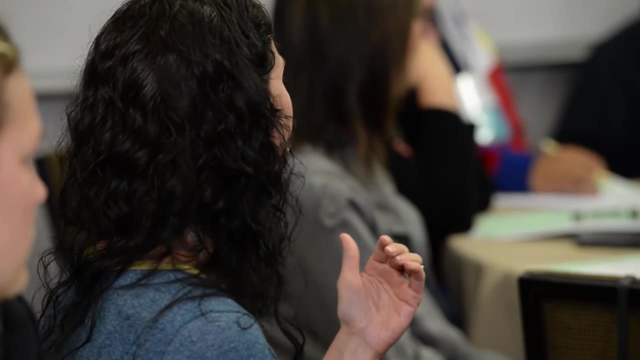 way the problem was originally given to you. We decided to specifically model a parent and child going on a college trip Thursday to Saturday and factor that into our cost. So we kind of focused the problem statement with the idea that later on we could modify that. 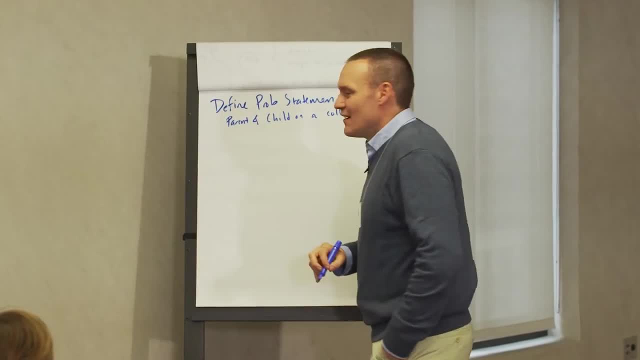 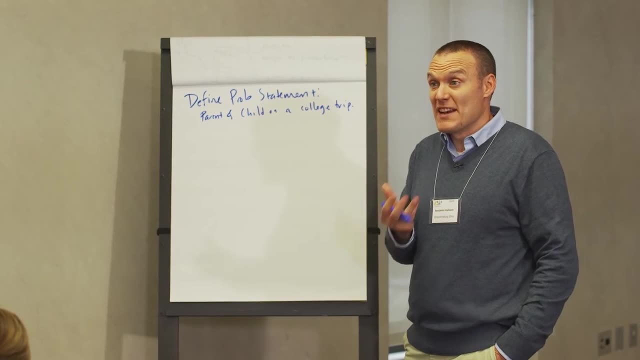 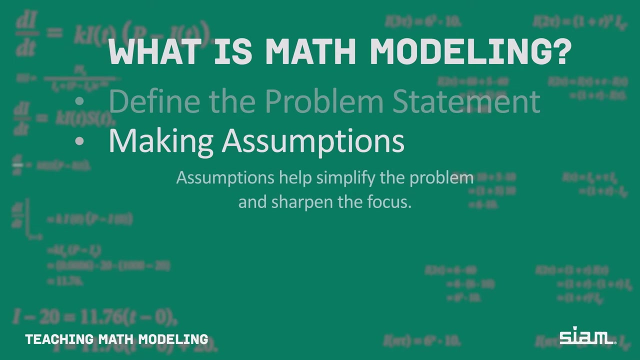 Right. And so, in doing that, what did you automatically do then? right, In defining the problem to be something that was more manageable. what happened? You made assumptions. You made an assumption, but it was something that made it tractable. right, You had to. 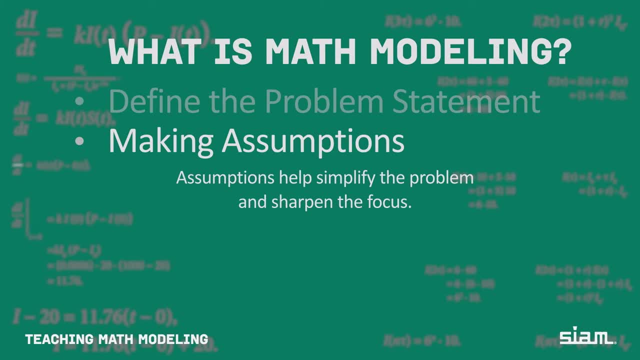 have something you felt like I want to see something- and maybe this is of personal interest, I don't know- right For someone in the room- or something that you could. you have students who are going to do that, right, Right, So they're going to do that. 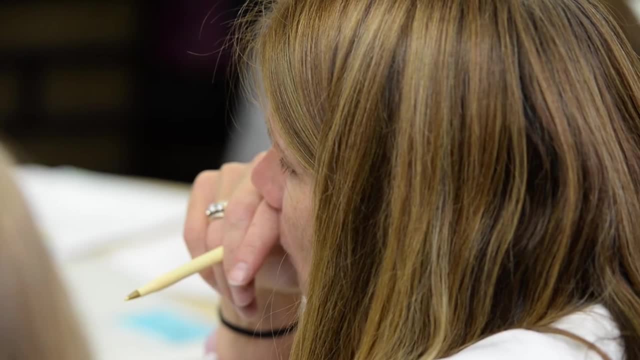 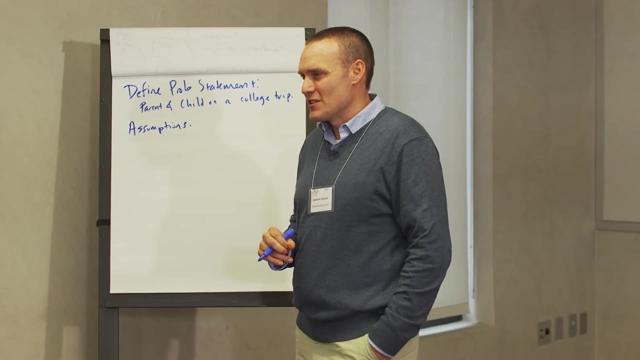 Right Right, They're going to go with their parents somewhere, And that makes a lot of sense. After you make some assumptions, what happened next? to try to solve the problem, Did you just jump right into it? What did you determine as variables? I think there's a lot of consistency in this. 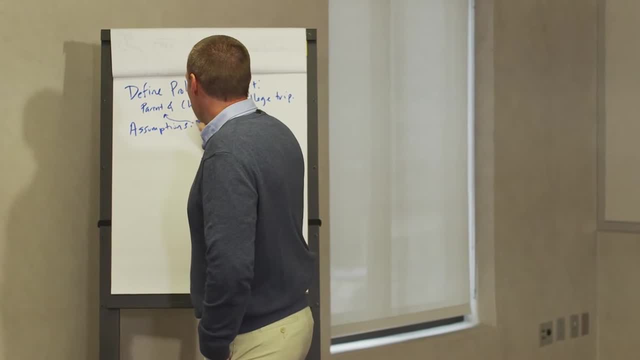 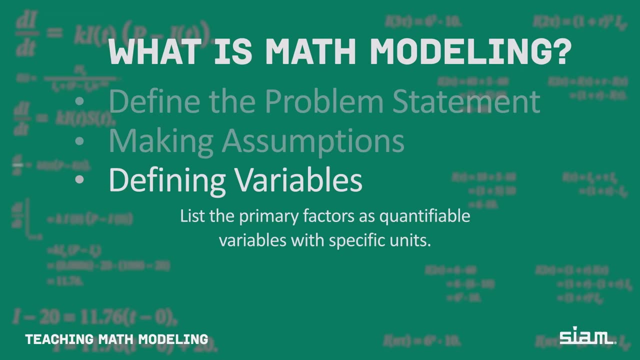 I'm going to put it down that we had some assumptions. We know we had these two things. There were a lot of other assumptions that took place, but we certainly had. we thought that these, like the time and the time And cost, had to be accounted for. And so I wonder here, right, If you're looking at 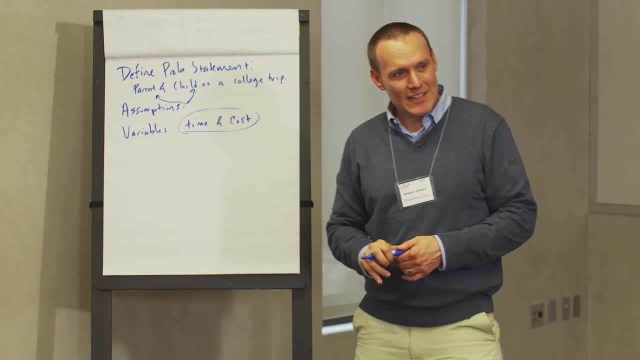 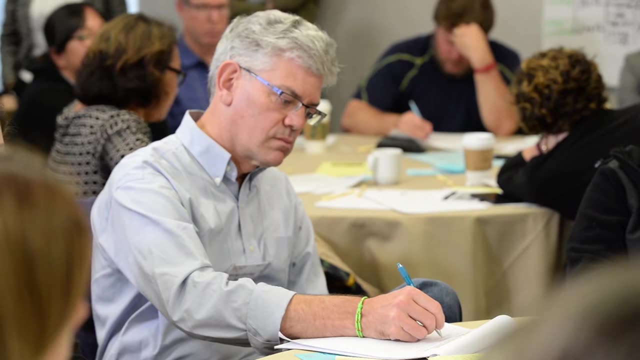 just time and cost. there's probably a number like you're. you're saying there's a number of ways. A lot of people were saying that they vary in terms of how we plug them into our model as we built our model. So I'll say a model exists because a lot of people had 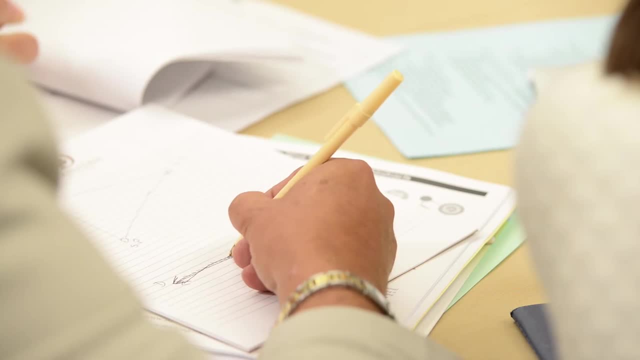 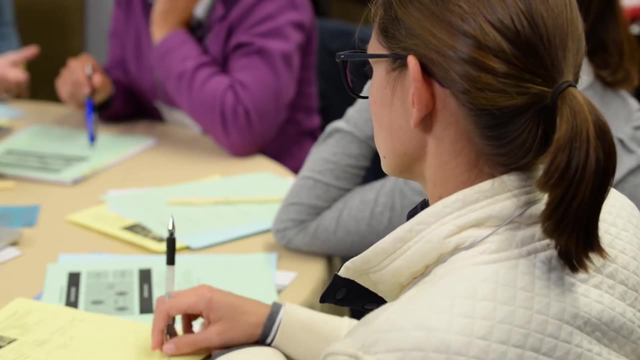 some sort of outcome which says: I basically have a total cost when you combine them together, And that's, I guess, trying to represent somewhat with the circle, When you combine those together. now we've made something different that, as we change that, we know we're going to have. 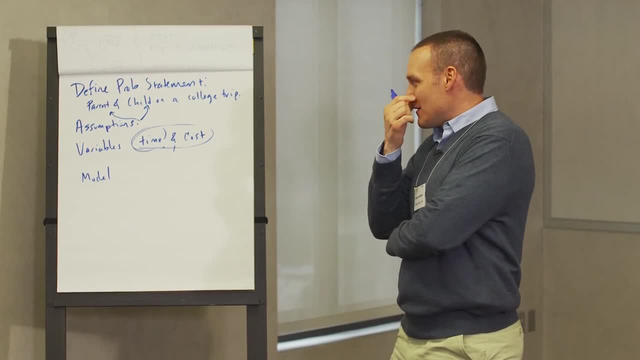 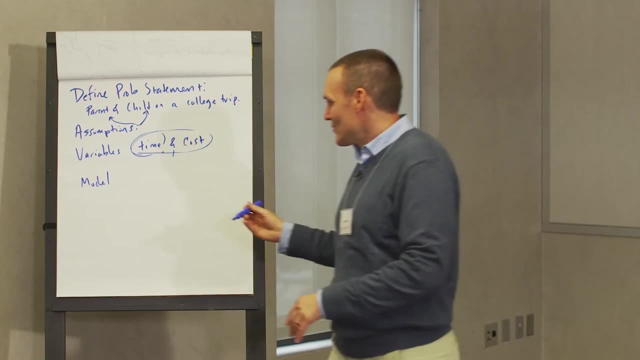 some different outcomes. So it's interesting to think of that as a variable or maybe a parameter that you're inputting into your model and seeing different outcomes right. So I might say, variable slash parameter. How do you choose to use that? You are plugging. 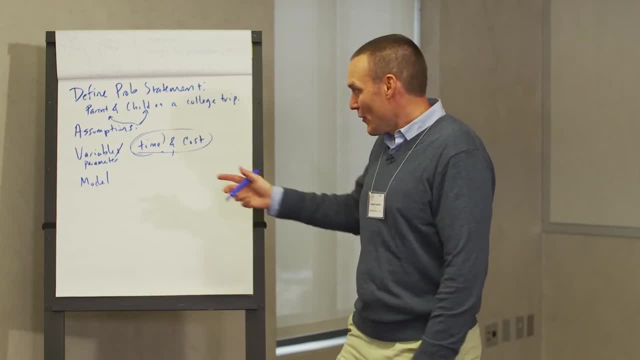 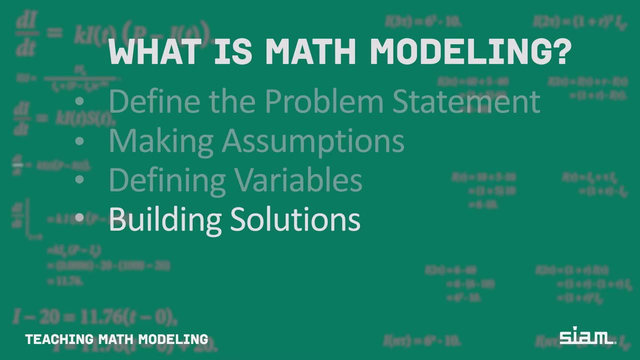 it into that model and getting some outcomes, but that already led you to a model because people got results right. So we have a model, We got solutions and a lot of them were dollar or time based right And dollar, time based. 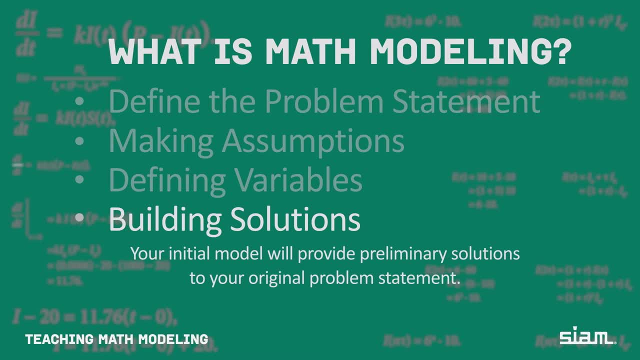 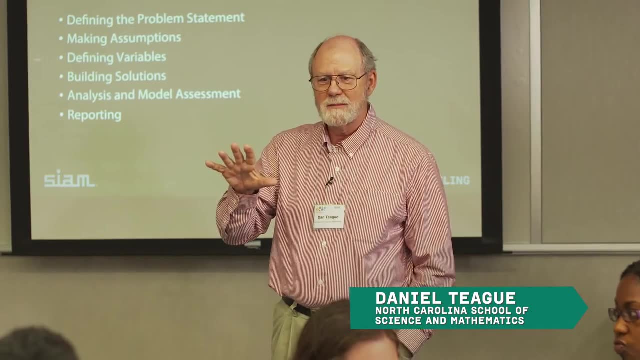 And I feel like some of the the the best ones. I know it's hard to get an answer in this amount of time. One of the difficulties students would have in a problem like this is there. there we'll look for some monster king function that combines. you know that that solves. 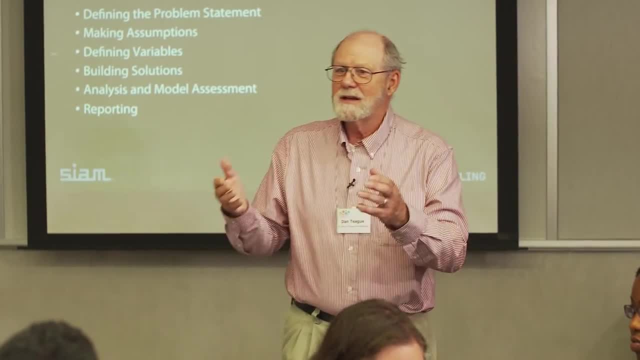 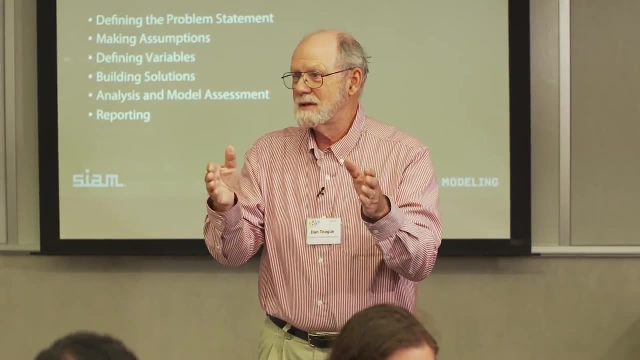 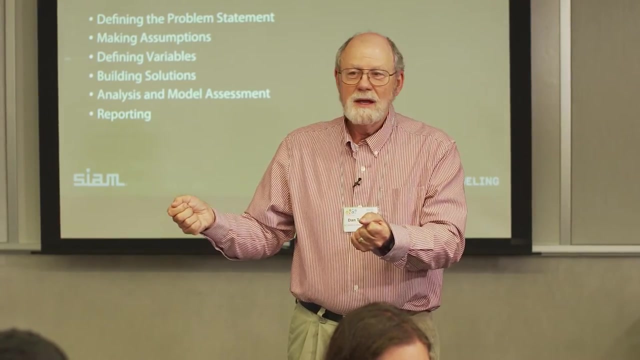 the problem because that's their experiences. those things exist And so it's very hard for them. And so you know we're going to look at this particular kind of trip, or we're going to look at a family trip, or we're going to look at taking kids, a group of students, on a trip. 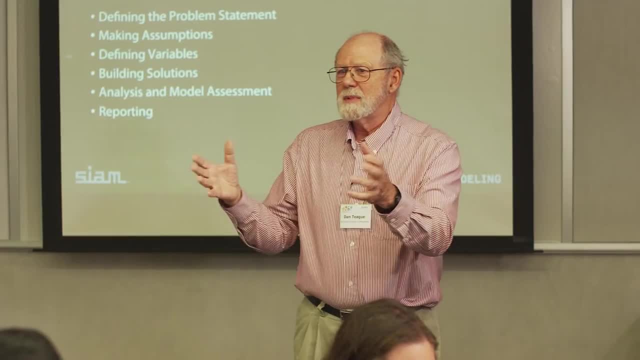 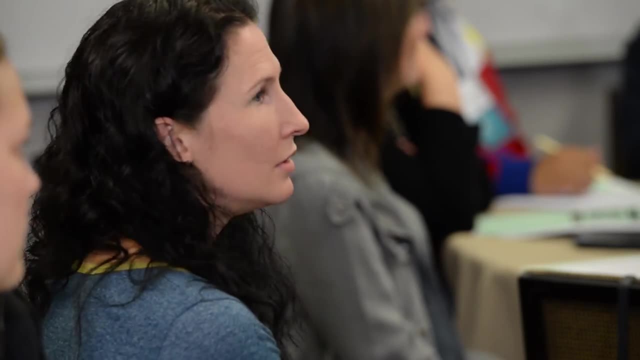 And one of the things that I talked with this group about is is you're going to be trying to mush several disparate things together- time and money, maybe coming up with a single value, or maybe you're going to have time and money as an ordered pair, Maybe the solution. 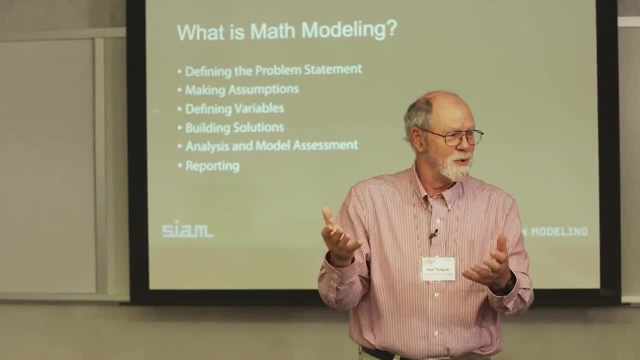 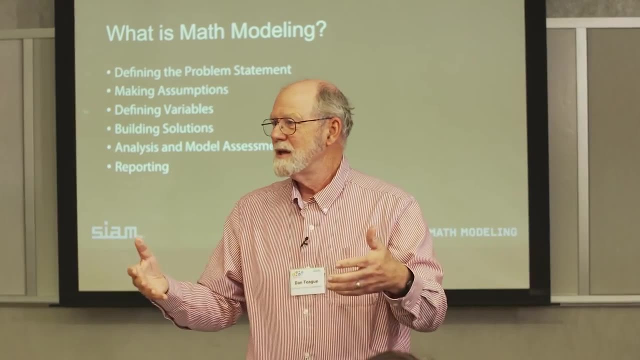 is going to be an ordered pair, a point in the plane, And then you get to the point where you get to look at the point in the plane and make some decision about it, But trying to figure out what you can combine, what are similar enough to put together And the expression. 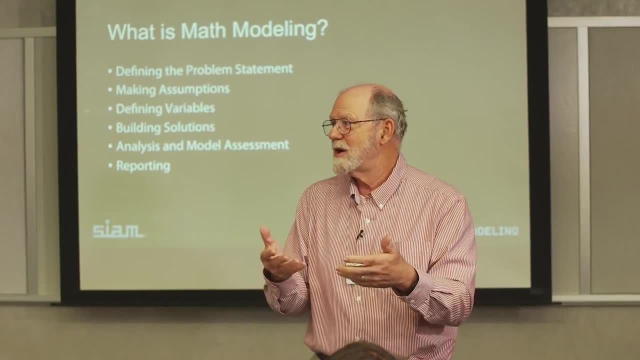 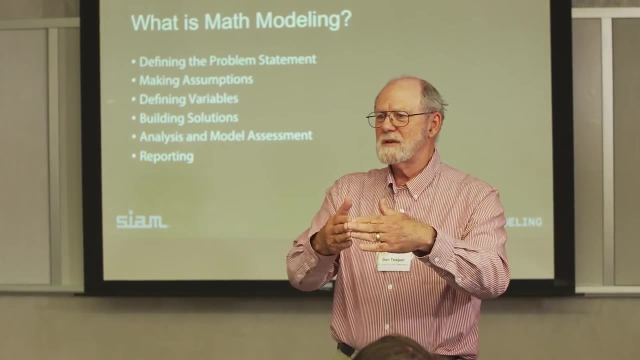 I use with the students is: it's okay to make a fruit salad out of apples and oranges. You can combine apples and oranges, but you shouldn't try to combine apples in Buicks. You know, there are things, some things that are sufficiently different that everything. 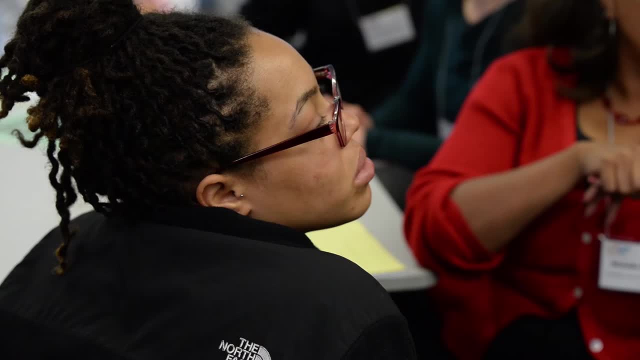 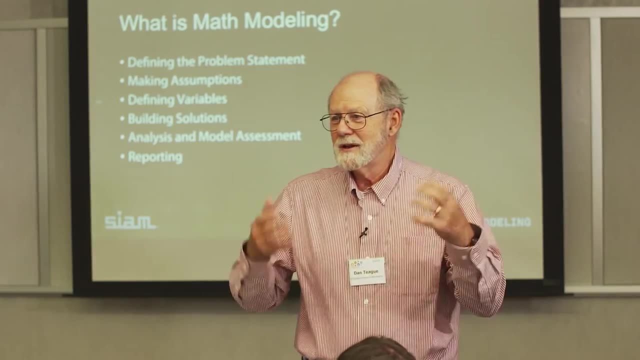 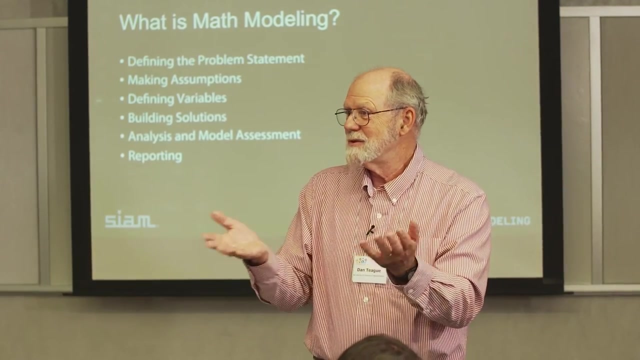 changes. Taking your debate team for a competition- Sorry guys, Competition might be very different than taking your environmental club for a conference on green gases. You might make very different decisions about how this group should be getting there, And those can't be rectified in a single solution. 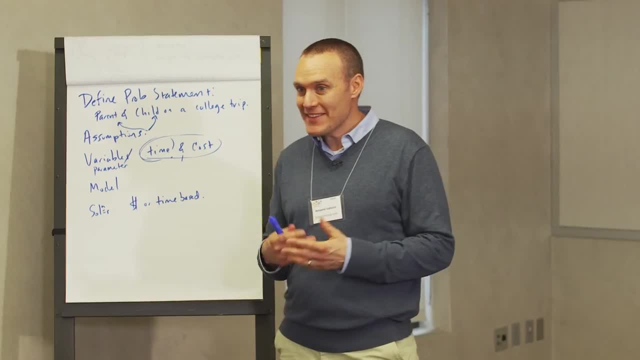 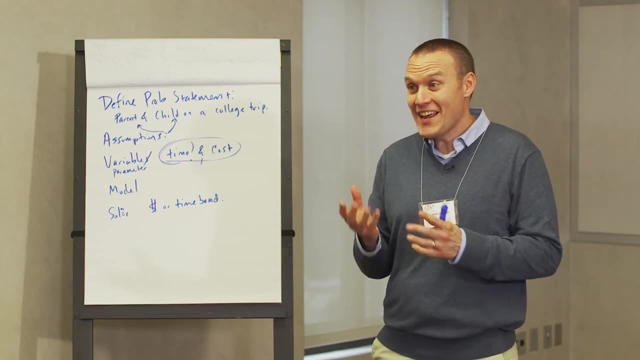 Once you get to this point and you're able to combine these different things, make the comparisons, And that's what I'm saying. So people in the same room have done enough different things. If you compare those things, you should have different answers for the same question.